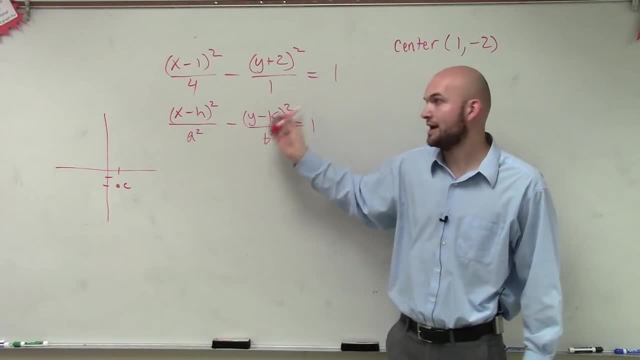 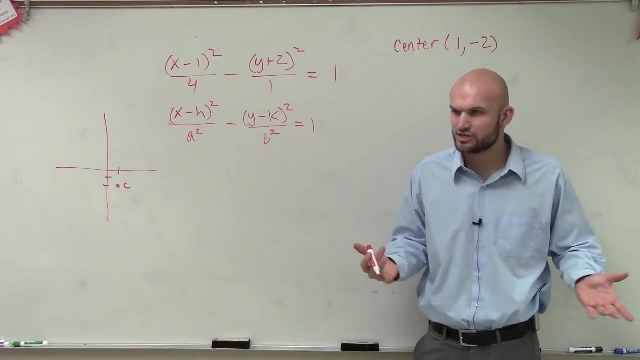 All depends on which coordinate is above your a. So, since my x is above the a, I know this is going to have a horizontal transverse axis. What is a horizontal? what is a transverse axis? The transverse axis is where your foci and your vertices are all going to lie. 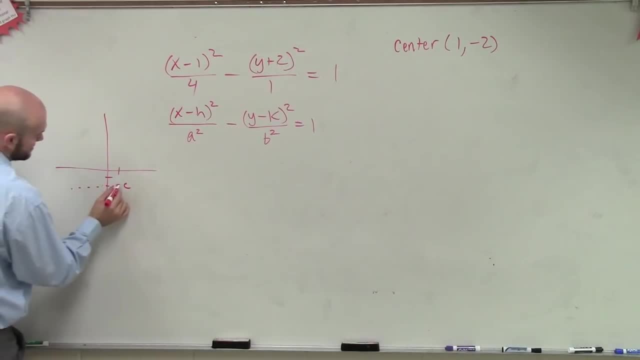 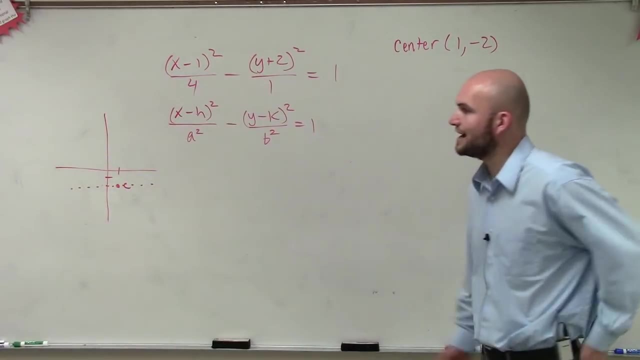 So that means they're all going to lie horizontally on this transverse axis. It's kind of like the major axis for an ellipse. All right, So to find our vertices. we know that the vertices, The vertices, are going to be a distance away, right? 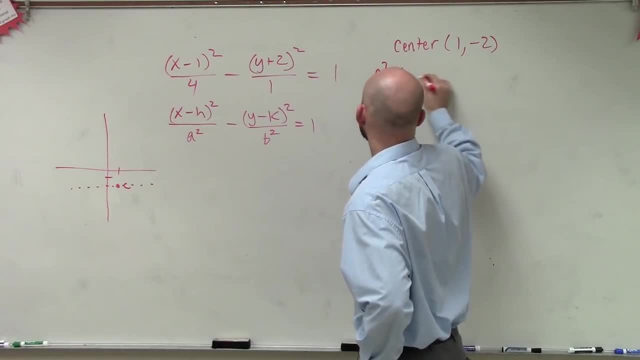 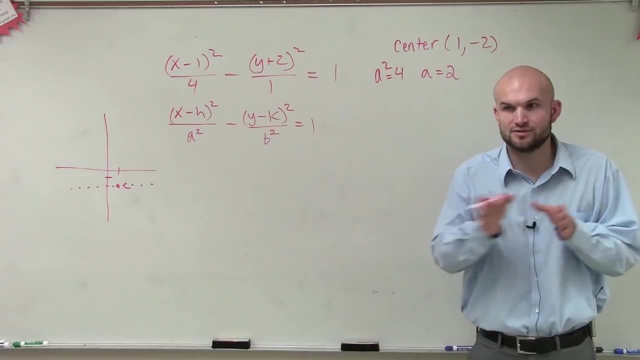 So we know that if a squared equals 4,, then we know a equals 2, correct? So that means from the center, my vertices are now a distance away. Well, since this is a horizontal transverse axis, am I going to add or subtract a? 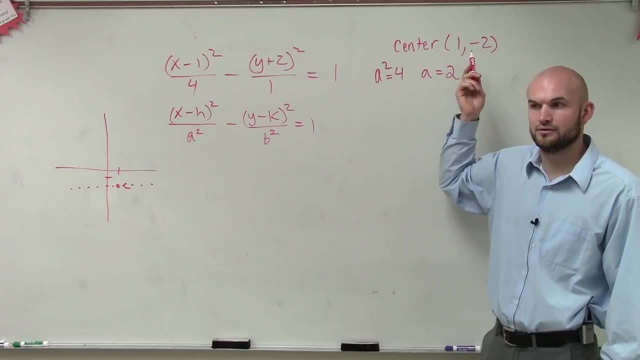 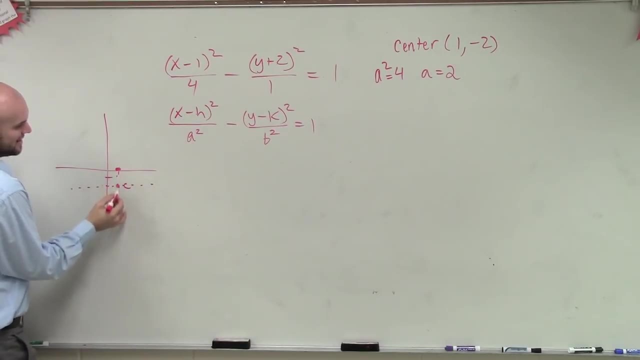 to the h coordinate or the k coordinate. H coordinate, Because when I add it to the k guys, I'm going to go up to And negative 2.. But I just told you it's a horizontal transverse axis, So you've got to add it left and right. 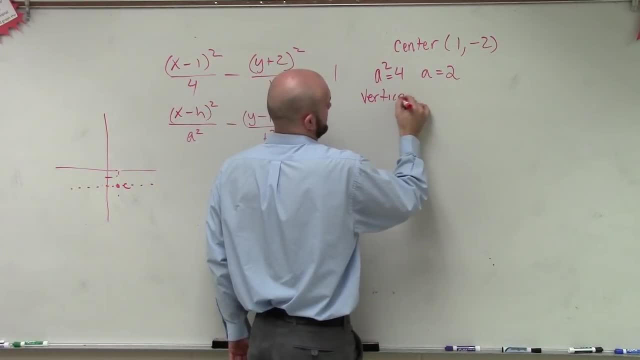 So, therefore, to find the vertices, I'm going to say it's going to be 1 plus or minus 2 comma negative 2, which is going to provide me with two vertices: 3 comma negative 2 and negative 1, negative 2.. 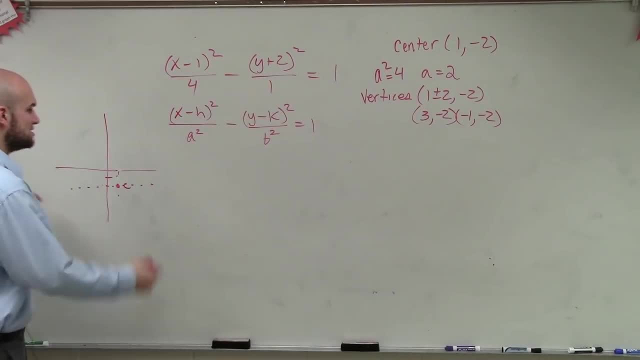 Notice how my k remains exactly the same. So now I'm going to have 1,, 2,, 3.. 3 is one vertice and negative 1, 3, is the other vertice. Let's put the c right here. 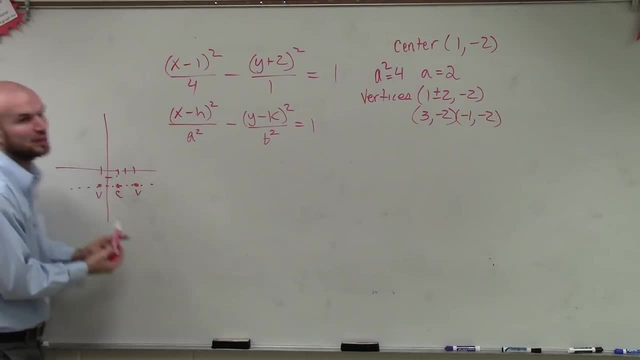 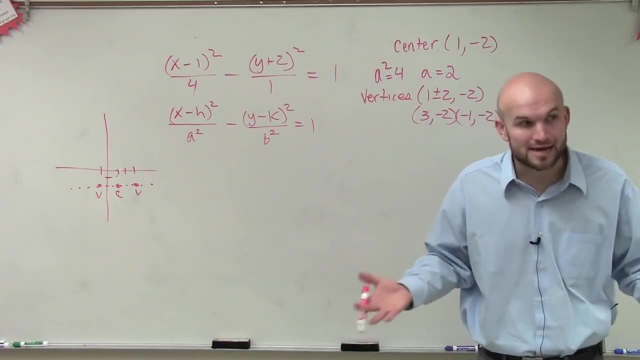 Do you guys see how the vertices and the center all lie on that same line? That's what we call the transverse axis. And guess what? The foci lies on what line? That same line, right, But now to find the foci. that is not a distance of a, not a distance of b. 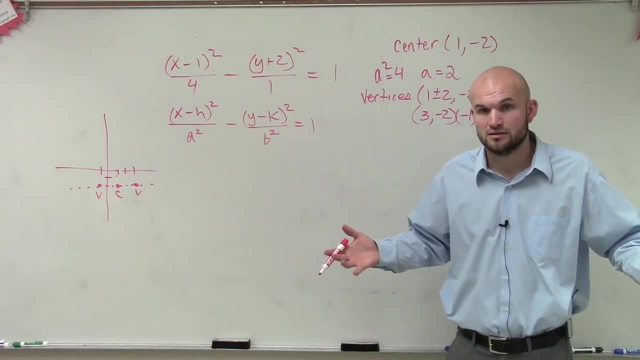 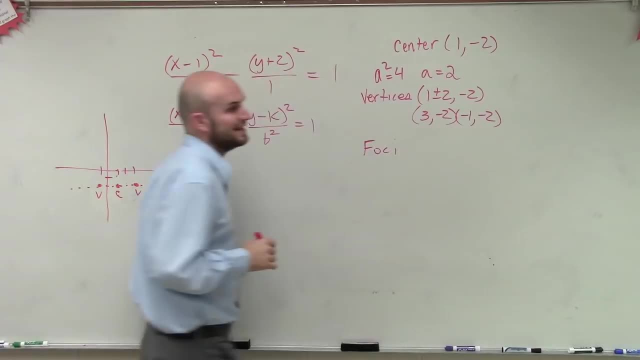 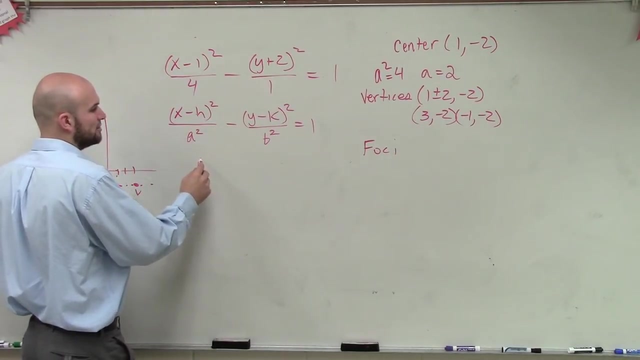 That's a distance of C, C. Okay, So To find the foci. now we need to figure out what is that distance of c? So we know for a hyperbola, to find the hyperbola, we know that c squared equals a squared plus b squared. 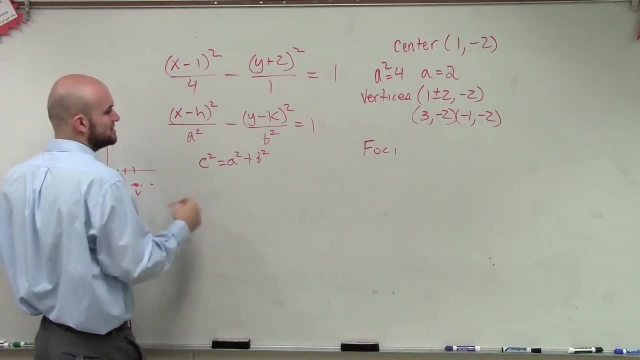 So hyperbola, we're trying to find out what c squared is. So we know a squared, we know b squared, So c squared equals 4 plus 1. So c squared equals 5.. Therefore, c equals plus or minus. 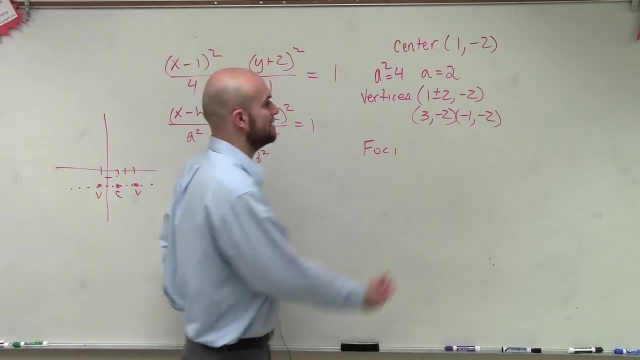 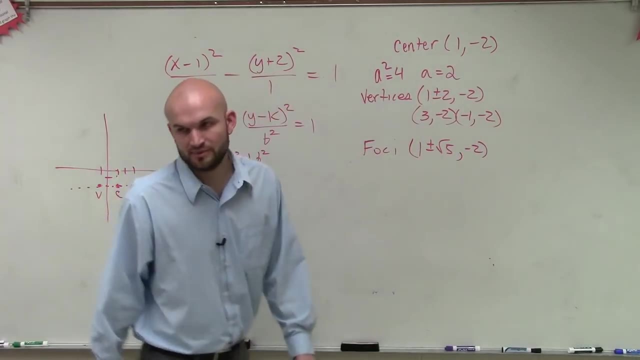 Square root of 5.. So now, what I'm going to do to find the foci, I'm going to do the same thing: 1 plus or minus the square root of 5 comma negative 2.. Now, I don't have a calculator with me, so we're just going to want to approximate. 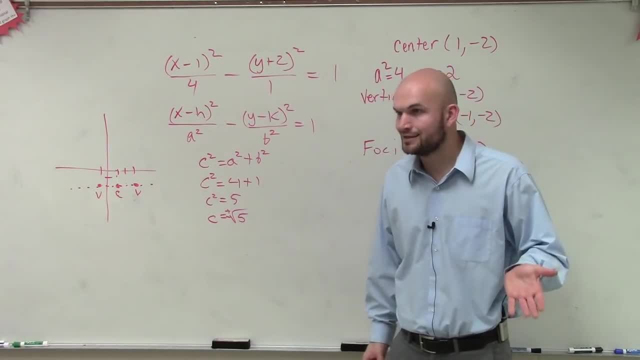 Well, if I know, the square root of 4 is 2 and the square root of 3 is 9, the square root of 5 is going to be somewhere in between there, right? So I'll just estimate it at like 2 and something, right. 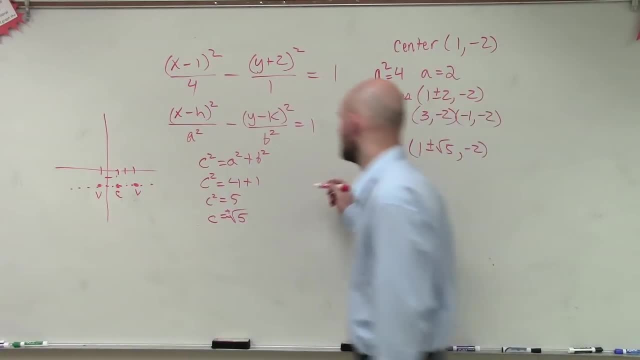 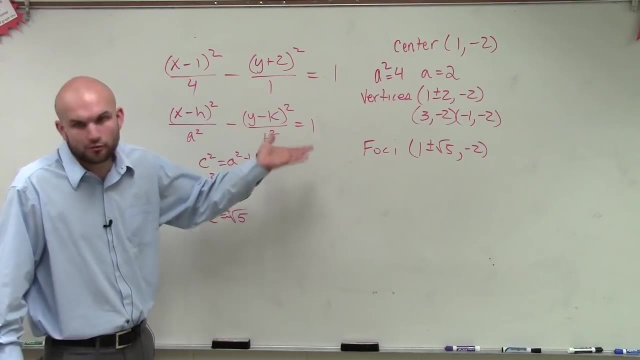 Okay, So. So let's say so. This could be approximated to 1.. Plus 1 plus 2 point, something would be like 3 point, something right, So I can add it over to 1,, 2,, 3, and somewhere in between there would be your foci. 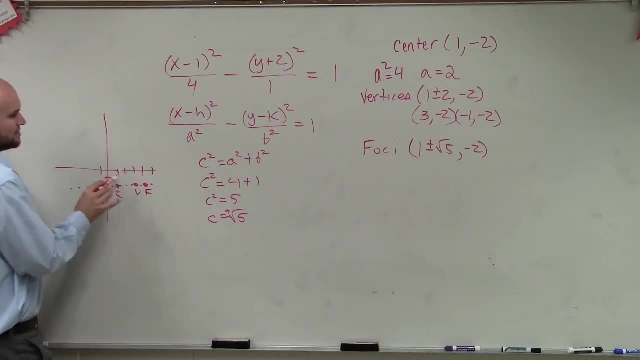 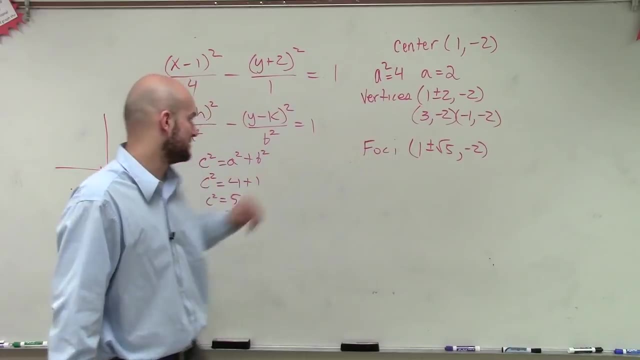 And then obviously, if you're going to calculate, you can approximate a little bit better. So now I'm going to subtract. So 1 minus 3 would be like minusing 2 point something. So now I'm going to go over 1,, 2, and a little bit extra. 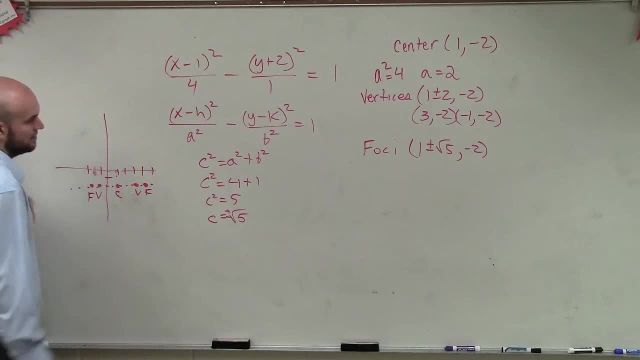 It would be somewhere right around there. So there's that foci, Okay, And again, I'm just estimating the foci. So now we know that my hyperbola is going to now go towards its foci. And they also asked us to find the asymptotes. 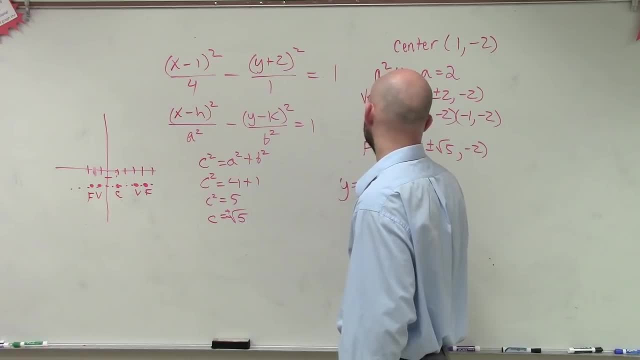 So remember the equation for the asymptotes is: y equals k plus or minus. Now, since this is a horizontal, we're going to have b divided by a, x minus h. All right, If it was vertical, your a and b's would be swapped right. 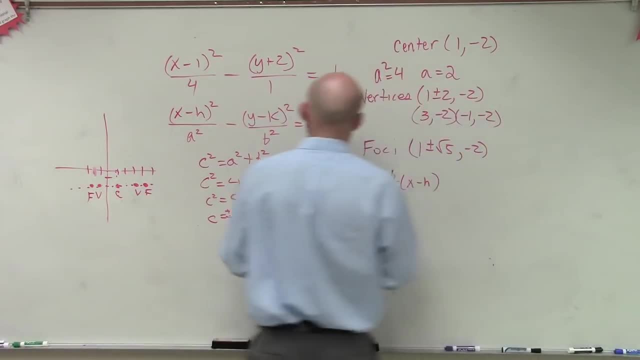 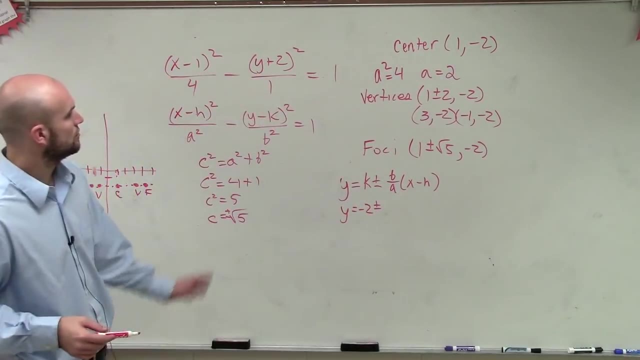 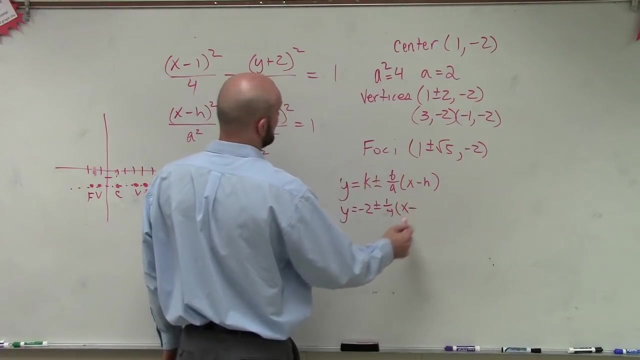 Yes, Two different equations. Okay, So now let's plug in our k, which in this case is negative, 2, plus or minus b, which is 1, over 4, times x minus h, which is 1.. Okay, Distributive property. 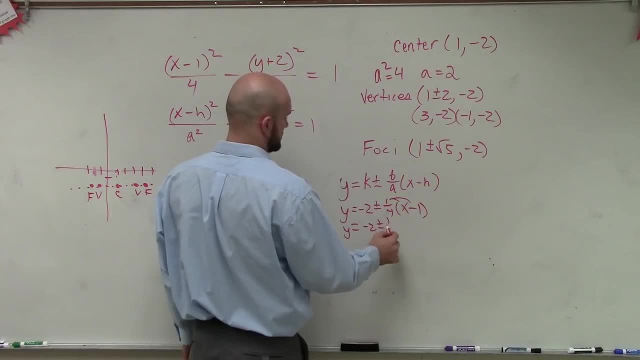 Y equals negative 2, plus or minus 1. fourth, So Isn't this over 2, though? What Isn't it over 2?? Oh yes, It is over 2.. That's it, Thank you. I was looking at a squared. 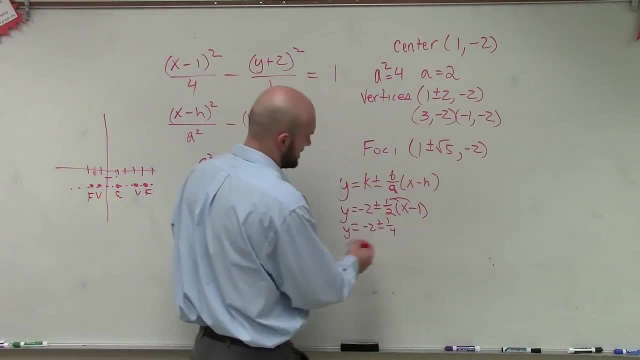 So one half. Actually. I'll just leave that. I'll just leave that thing So darn. I'll just go through this, Okay. So what you guys can see is, once you distribute that, then you can go ahead and have your two equations. 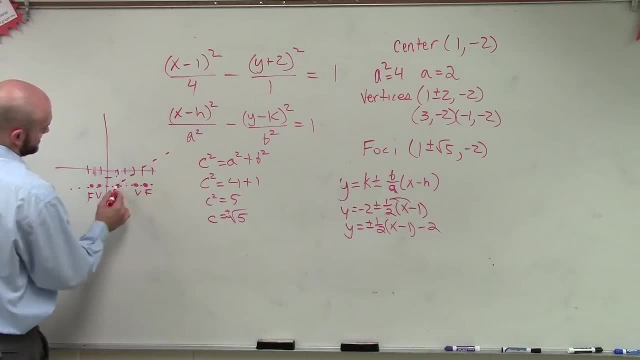 which are going to produce your two asymptotes, which is going to look something like this: So you're going to have two different x-intercepts and then you can sketch your hyperbola. Does that answer your question as far as on your foci? 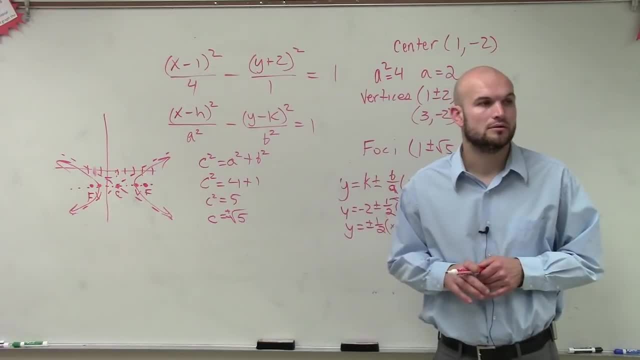 what it's going to look like and go for it. And when we're sketching that asymptote, can we just like estimate? Well, no, you're going to want to find what those exact equations are, So let's go ahead and distribute this out. 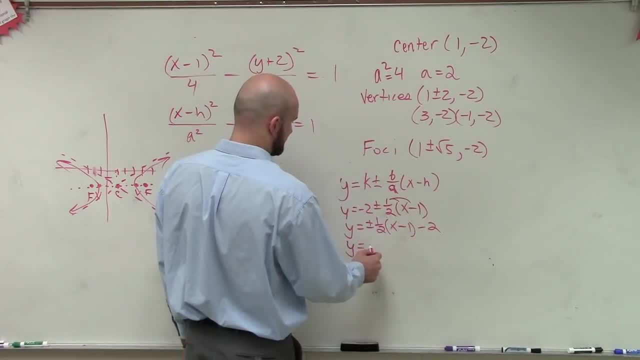 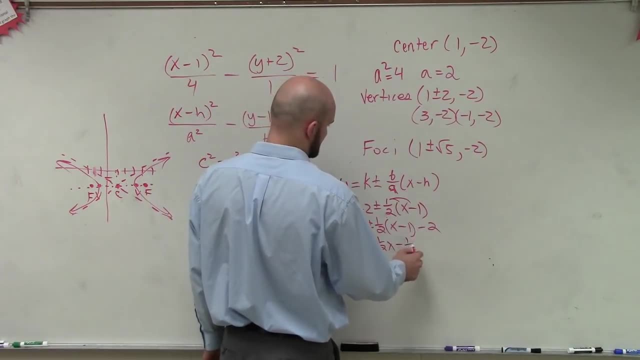 So I have: y equals this is going to be plus or minus 1 half x and this is going to be minus 1 half, And then so you can multiply. So let's just do it as two different ways, Okay. 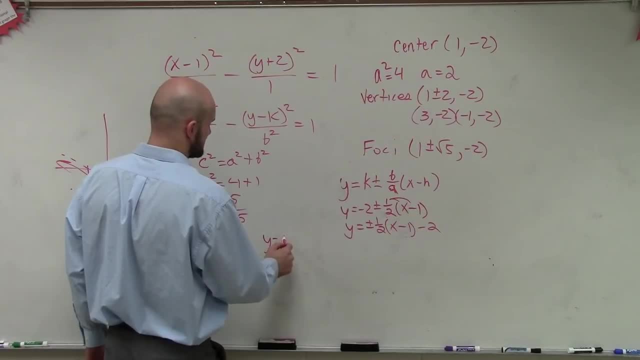 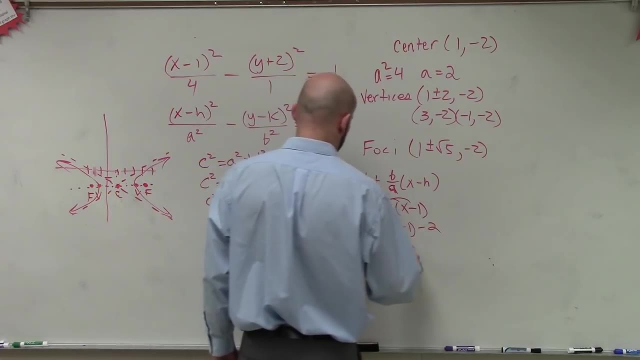 So you can do plus. you could have y equals plus 1 half times x minus 1 minus 2.. And you can have y equals negative: 1 half x minus 1 minus 2.. Right, You can do the positive and the negative. 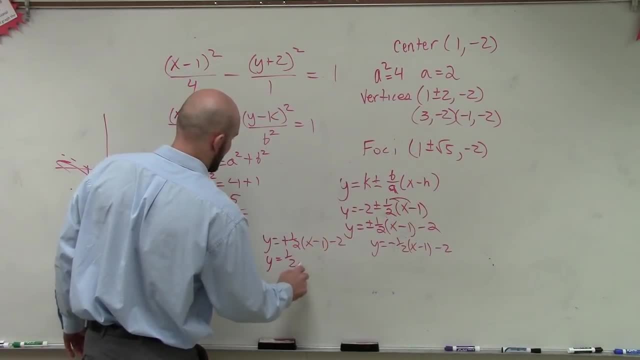 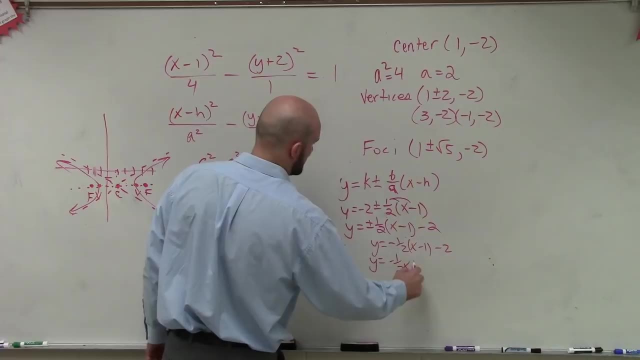 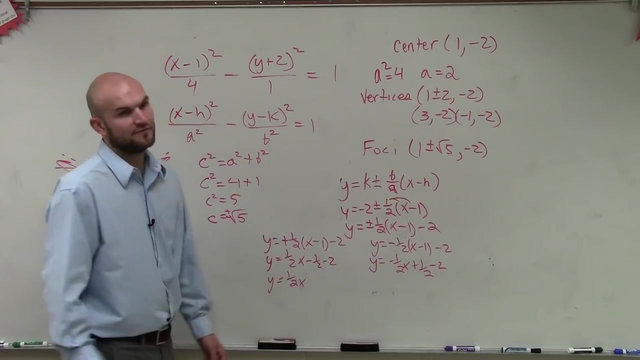 So if you did the positive, you get y equals 1 half x minus 1 half minus 2.. And here you get y equals negative 1 half x plus 1 half minus 2.. So in this case you have y equals 1 half x negative, 1 half minus 2.. 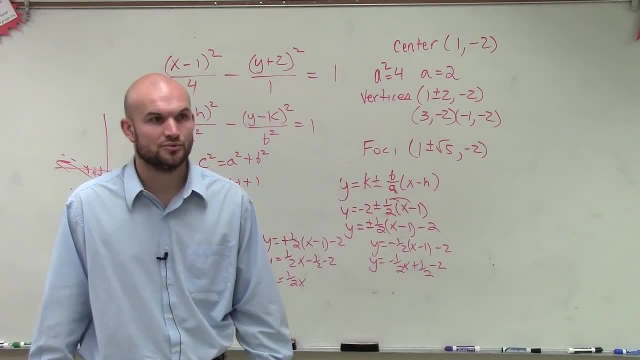 You have: y equals 2 plus 2 minus 2.. So this is going to be like negative 2 point 2.5.. Which would be the same thing as 5 halves, Right? So it would be minus 5 halves.